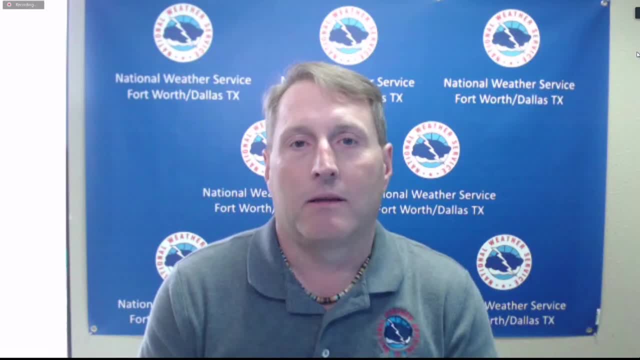 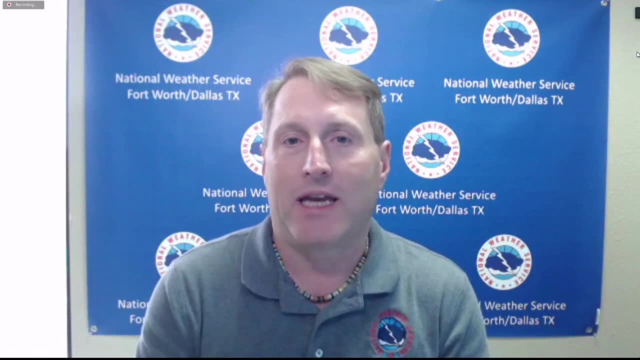 with the rivers in our area. The easiest way is to break it down into mathematics, and we use political analysis to determine the percentage of rainfall that is burned into the ground, and then we estimate the percentage ofпервых which percent of that volume of rain. 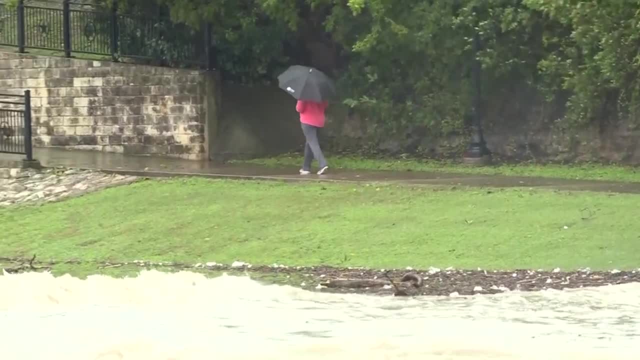 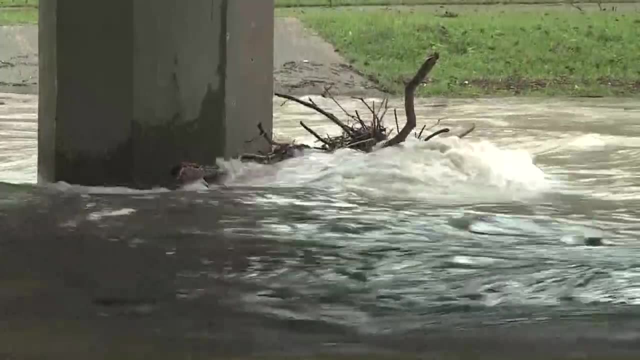 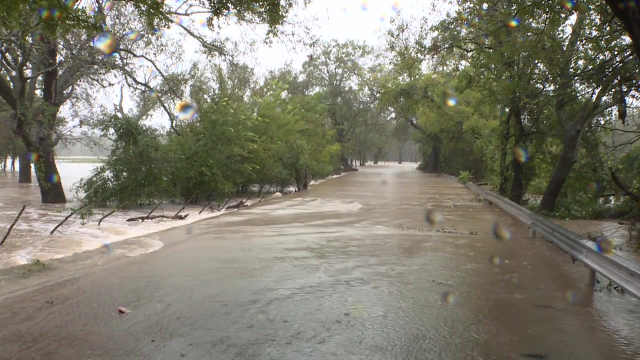 soaks into the ground and what percentage runs off. We now have a volume calculation of runoff. We then try to estimate timing, runoff response and routing responses, and we rely on federal partners to give us data so that we can figure out a volume and flow of rain relative to the amount of rainfall that is burned into the ground. 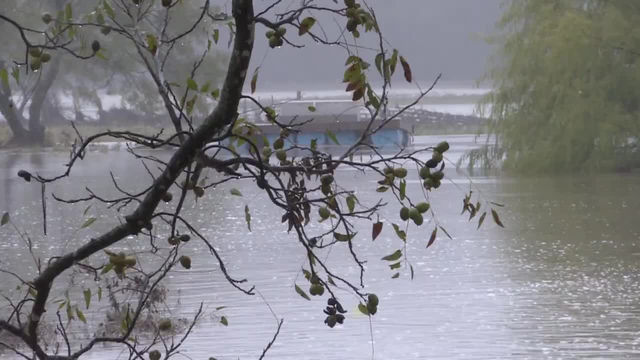 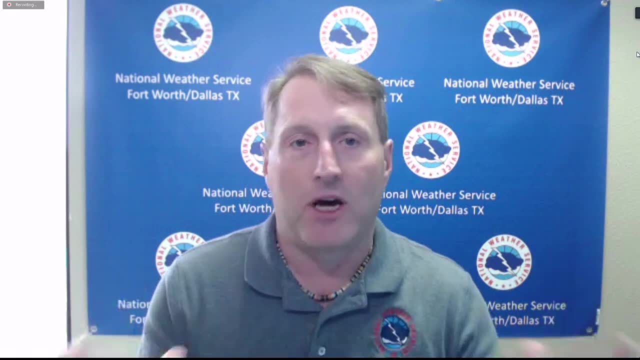 into a height measurement so that you know river at 28 feet. oh, I know at 28 feet. I need to start taking action. so there's a lot of math, a lot of science, but just think of it, as there's a volume of water coming down, how much of it's? 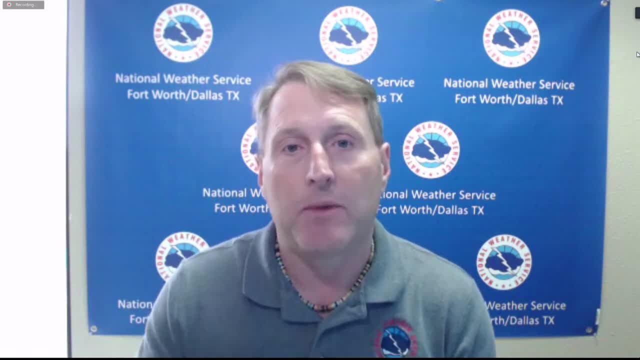 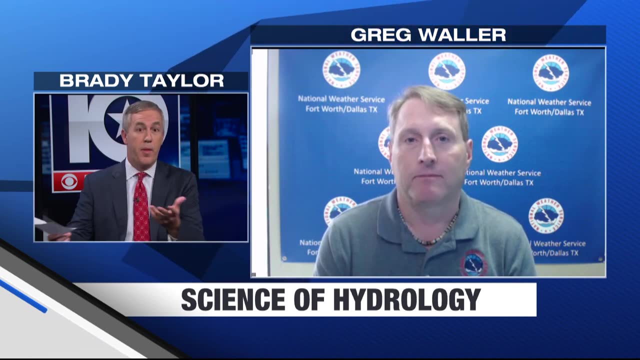 going to hit the ground and run in, how much is going to run off and then the timing of draining it downstream. so I know in meteorology we use models for a lot of stuff. how much modeling do you all do, with all the math and science to? 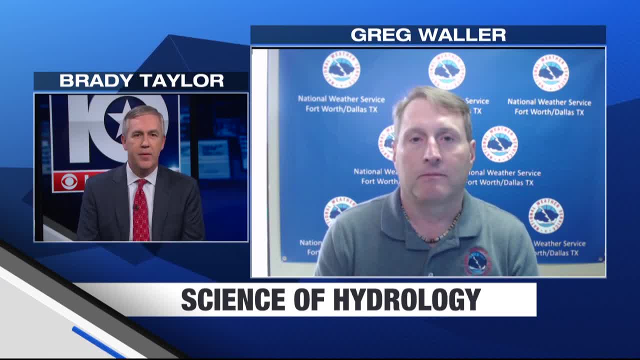 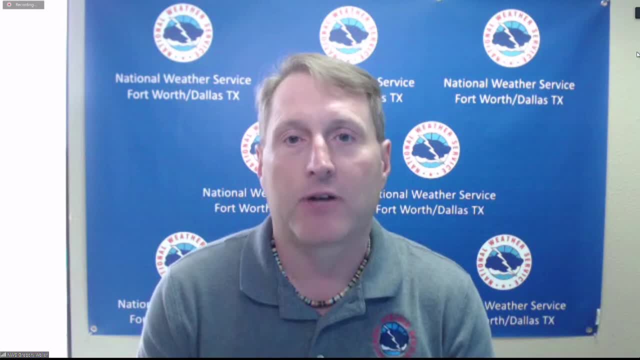 try to figure out how these rivers are gonna rise and how the water is gonna affect everything. a lot of models we use one primarily, that's a, a mathematical, it's a hydrologic model. but we, with computing technology increasing, we have multiple model sets now that we can use. we can use more physics and dynamics. 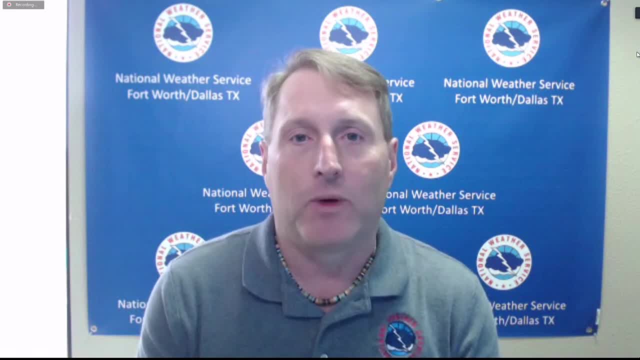 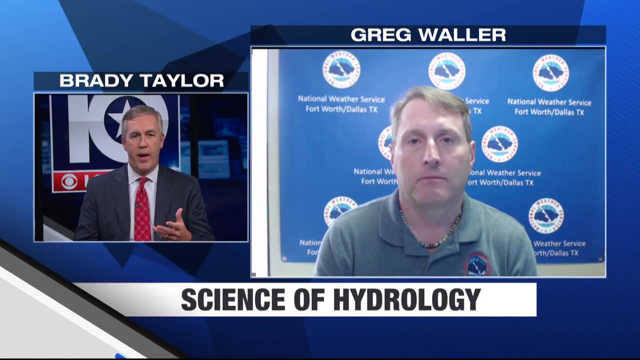 based models. it's like give us a scientist, give us data. we love it. we use one operational, but we'll look at others to help us fine-tune our forecast. so when we talk about river flooding- which is a lot which I'll do for the viewer- 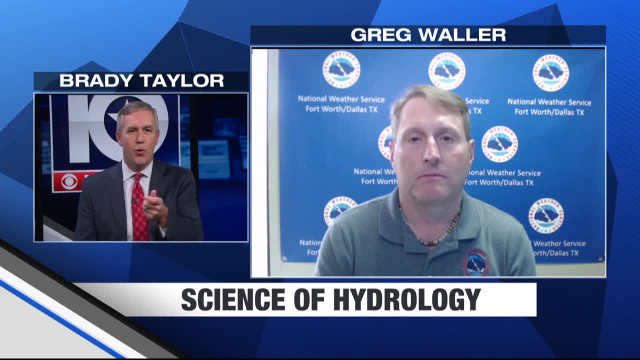 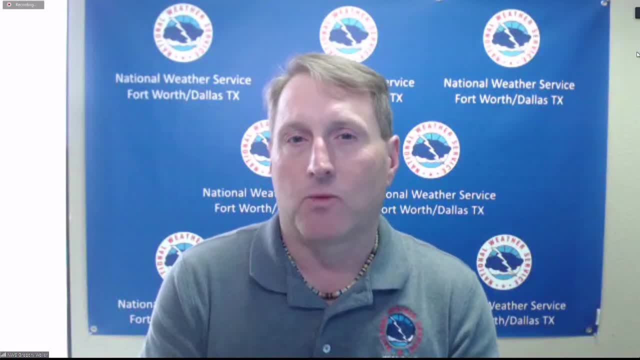 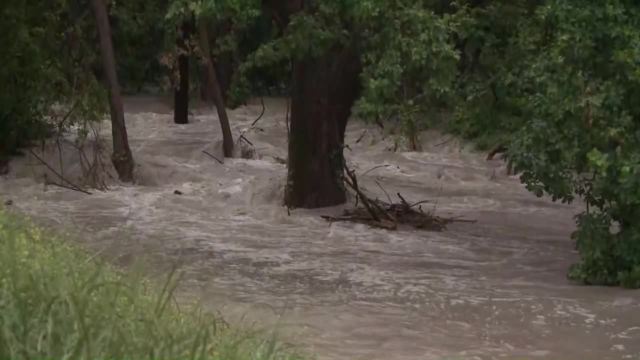 out there. what's the difference between the river flooding and the river flooding that you are trying to forecast, for it's an area that overlaps. the easiest way is that if it is associated with the river rising, that is river flooding. heavy rain can produce flash flooding can overwhelm storm drainage. 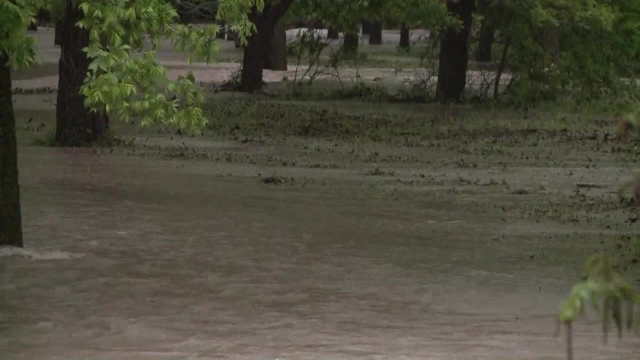 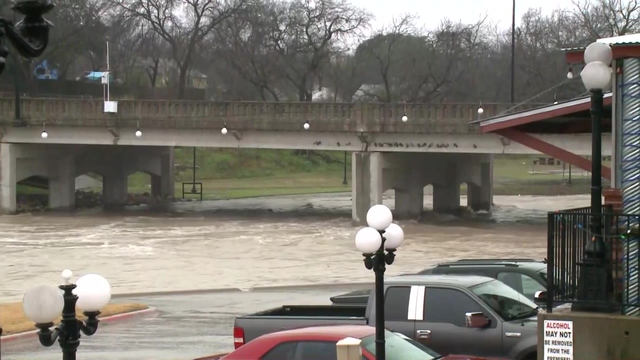 and can produce aerial flooding. that is a short term. eventually it makes its way to the river and then the river starts rising. so the weather forecast offices across the the nation, including the National Weather Service here in the Fort Worth. they will issue flash flood warnings and those type of products to. 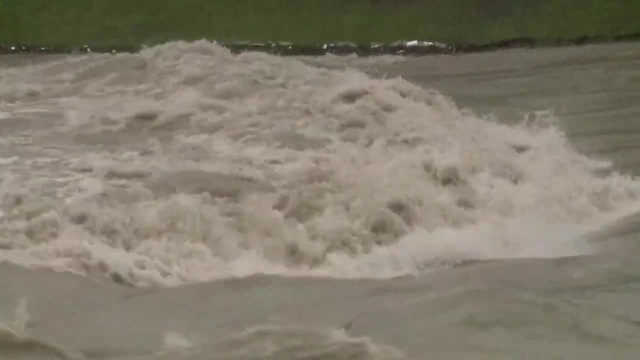 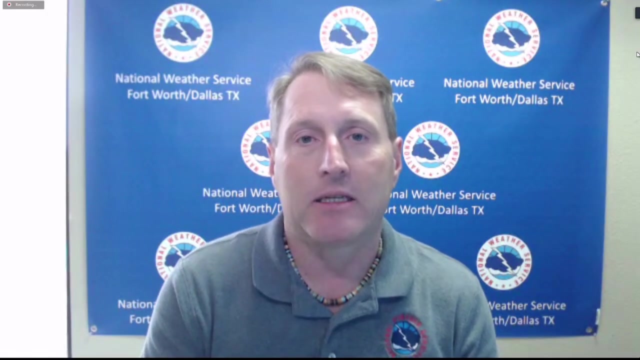 cover the short term and the aerial, but once it gets to a river system, we call it riverine flooding. then it falls, the calculations fall under the river forecast Center and we provide guidance so that our weather offices can issue more products that are more fine-tuned and detailed to help people make. 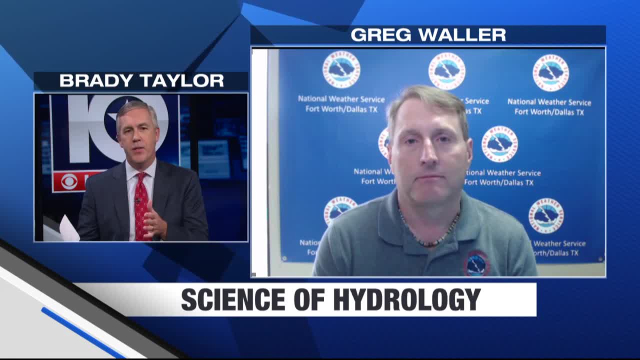 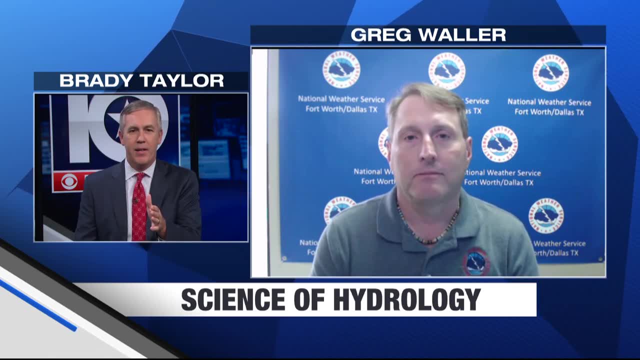 decisions. so you were talking about a volume of water coming down. how hard is it for you when you know you're talking about soil, how moist it is, but also the, the urban impact of that, of you know concrete, and all that of how, how much does that? 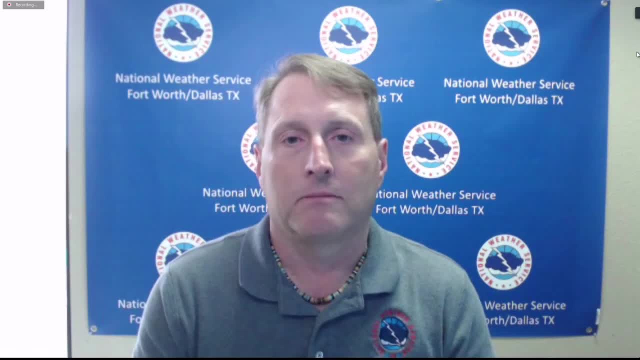 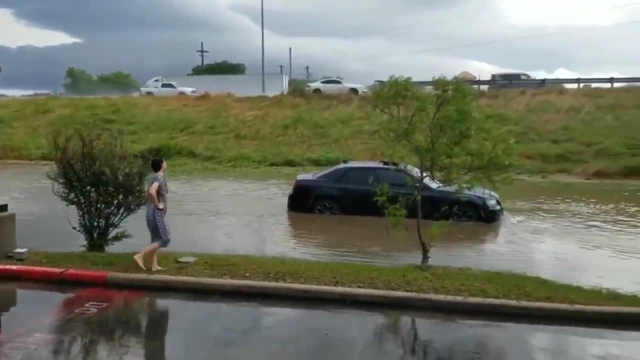 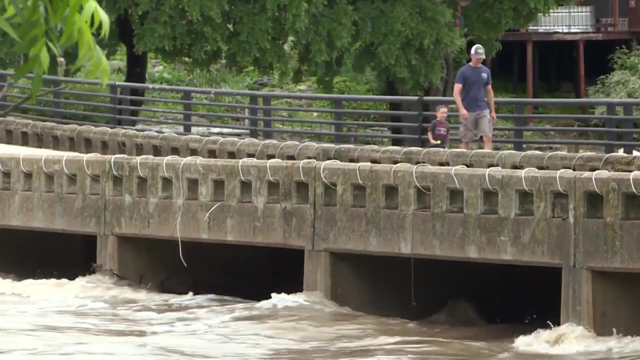 affect runoff as it gets to the rivers, and the flooding concerns a tremendous impact because if you take an open field and put a subdivision with a strip mall, you've now increased the impervious area of rooftops and concrete and made it run off a lot faster. so we are constantly having to recalibrate our models because we we try to. 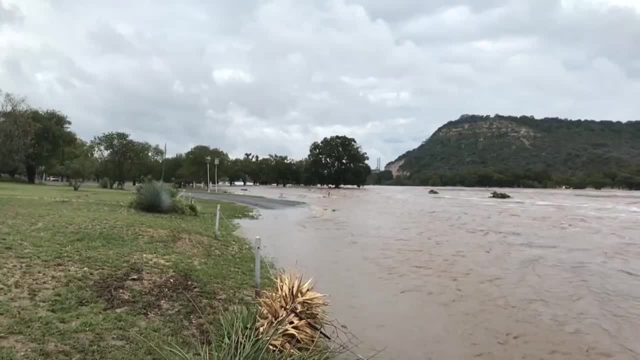 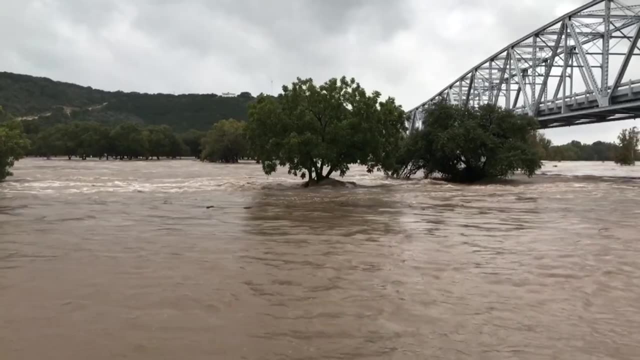 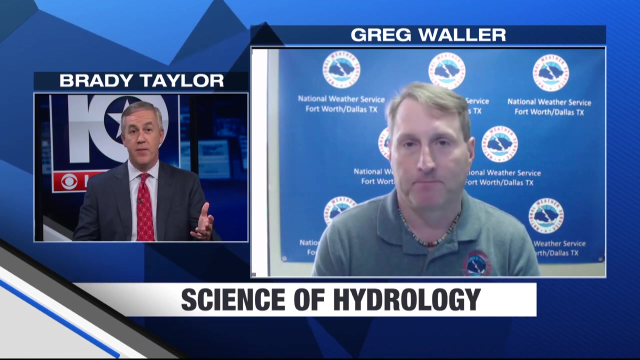 simulate land use and if something changes then we've got to go back and calibrate it. recalibrated to know more runoff and faster runoff, uh, to to then put those calculations into our river model to try to predict river health levels. so we've got a lot of major rivers that run through the 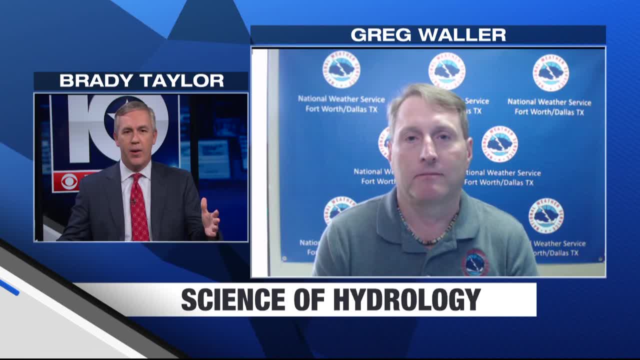 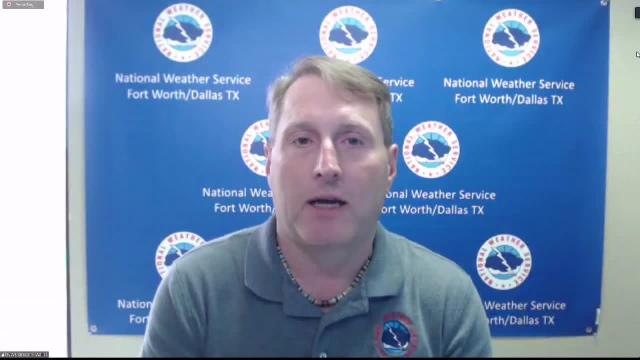 state of Texas to explain how big of an area y'all are monitoring and forecasting for with these River basins, our forecast area of responsibility. I call ourselves the Texas River forecast Center, but we we don't handle the sulfur, the red or the Canadian. we are the. 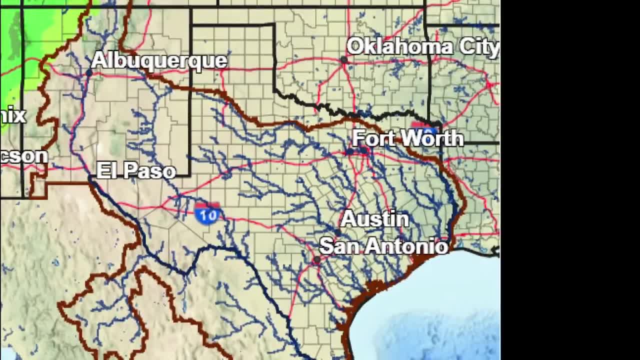 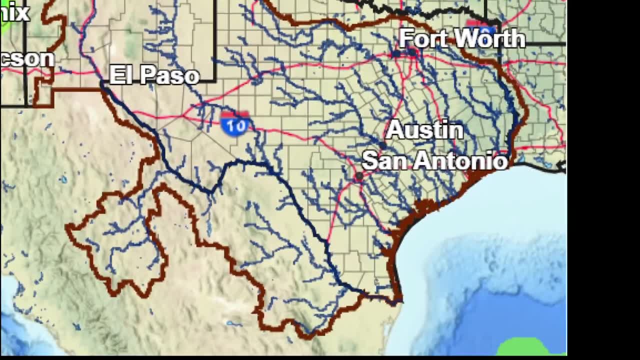 Sabine River on the Texas- Louisiana border over to the Rio Grand and we are the responsible agency for the Rio Grand flooding. so that is a a multinational, you know aspect. there it is over 400 000 square miles and if you think about, you know the the. 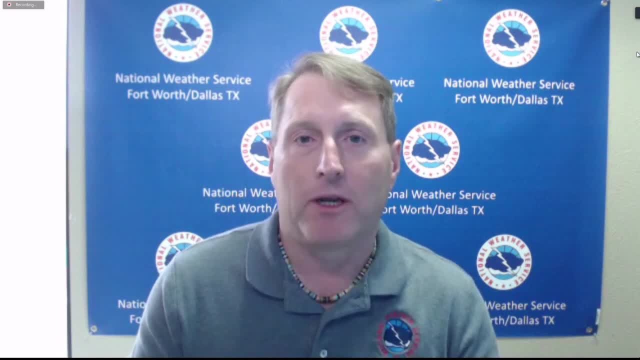 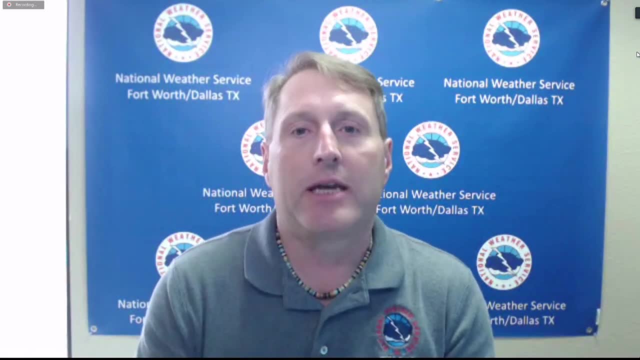 large area. you know every Lake that's been built. and think about that for a minute. the Texas only has one natural Lake and it's not in the River forecast centers area, it's up in in Northeast Texas. each Lake that has been built: you need to know why it was built, who owns and operates it. 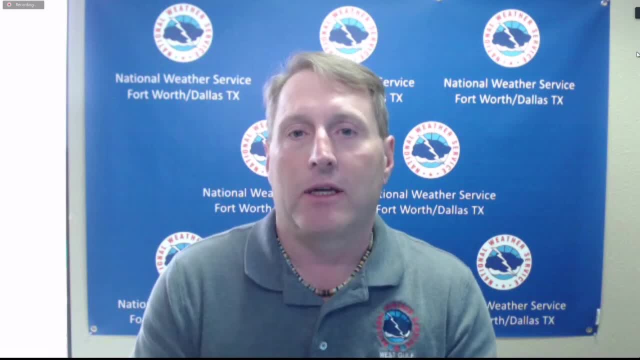 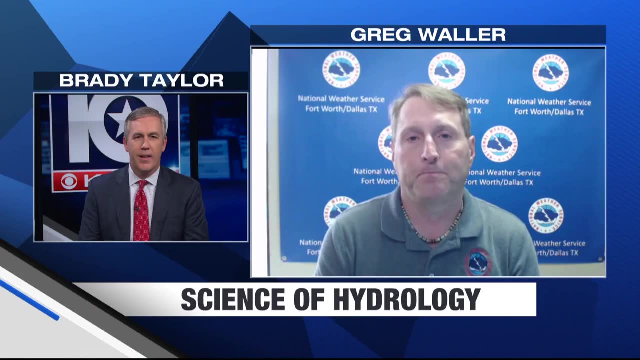 and the owners so that you can coordinate releases. so it's a. it's a large area of Footprint, uh, and then there's a lot of moving parts and moving pieces of people you need to coordinate with. yeah, that's got to be. yeah, there's a coordination of. 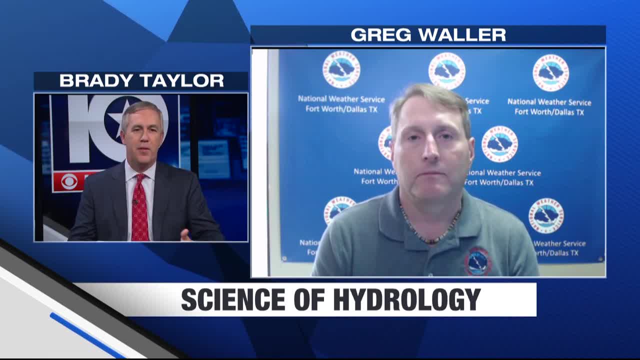 this got to be amazing with it. so you know we're talking with you on flooding and a lot of people are like, hey, we're in a big, bad drought, but uh, how, how does this drought affect y'all's forecast? when you start talking about the potential of flooding when we do get a big rain event. 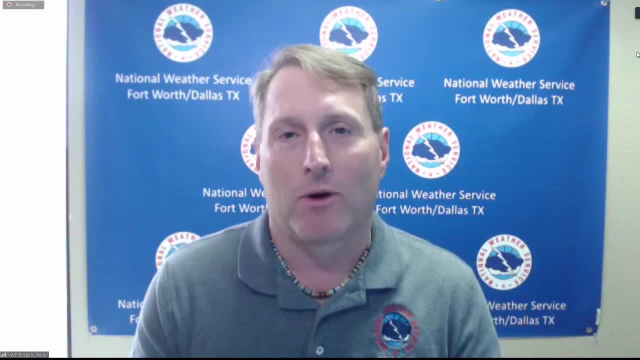 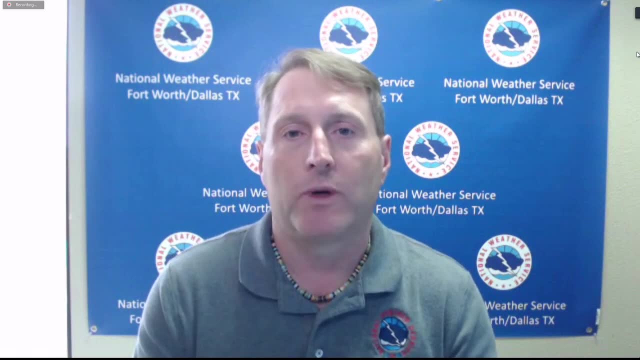 normally, you know, we would joke that if it ain't, we ain't working. that's not the case. we are always doing model calibration, flood inundation, mapping, calibration. we're doing extra work. so when it stops flooding we're still very busy, but during a drought it goes into another one. in that water deliveries, we assist the river. 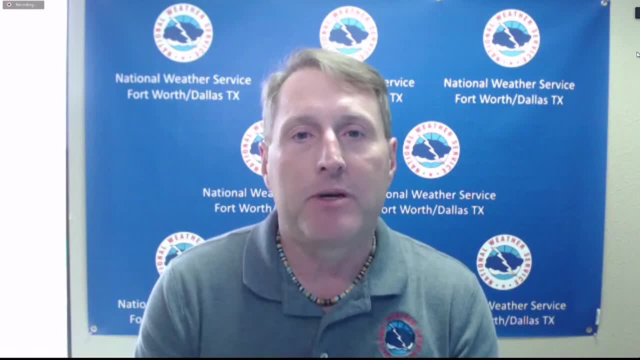 authorities and other water. you know water agencies to help them make decisions on their releases so they can meet their contracts. so we have weekly coordination calls with the large operators across the state to help provide them guidance so that they know what to make on Low Water deliveries, and it's almost as critical as it. 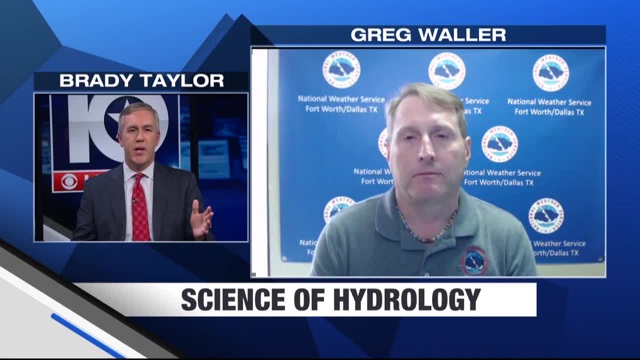 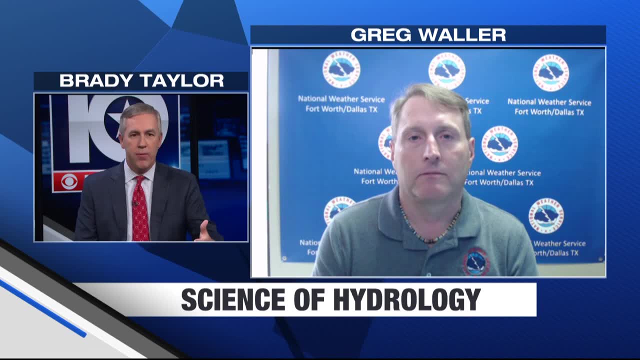 is when there's high water and Flooding going on, so you cover a large area. is there certain rivers or portions of the rivers across Charles forecast area that y'all really get more worried about, that become more flood prone or can affect more people? that's a good question and it's kind of double-sided. as you go from east to west you go from a literal swamp in the Subin river area more rain out east, so we focus on the rainfall aspects there, but really it's the impacts we're really concerned with the metropolitan areas: dallas, fort worth, all the entire i-35 corridor. 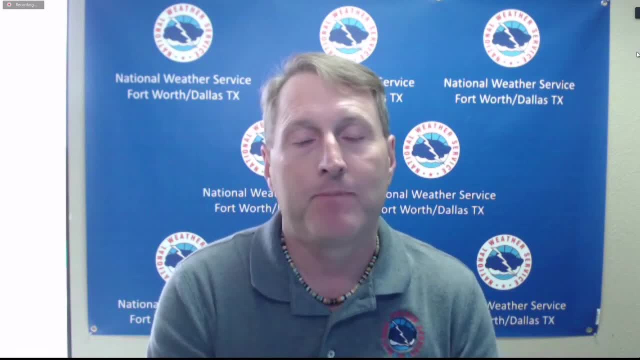 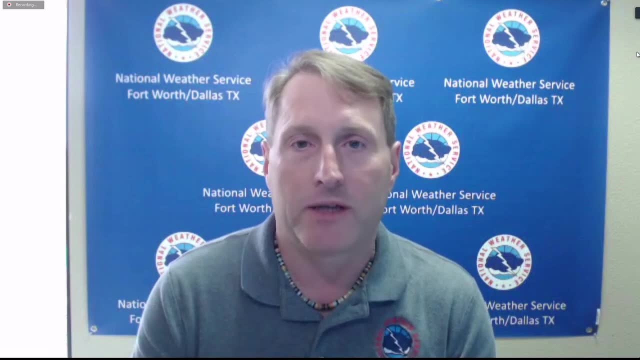 down to austin and san antonio, especially with the buildup that's occurring in that area, and then the coastal areas, houston, corpus and brownsville. the metropolitan area is there. so you could say the trinity river is important, the brazos river is important, you know the guadalupe, san antonio. 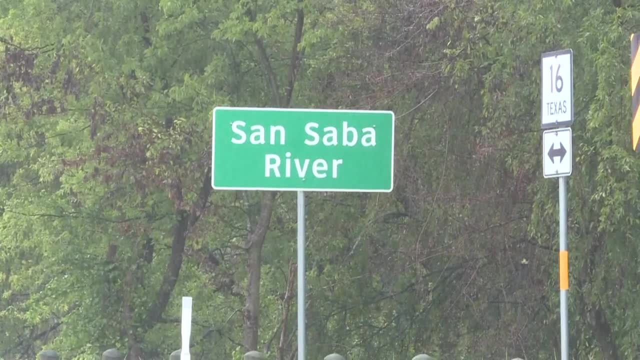 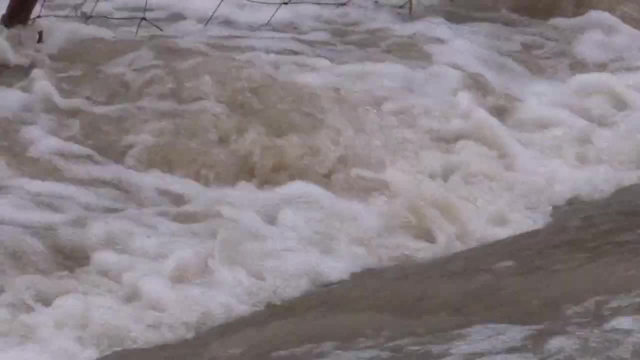 san jacinto. but in actuality, all rivers are important because, as mother nature just taught us, a heavy rain event can occur anywhere in the state of texas and you better be ready because there's a different vulnerability with each river system. we may look towards the population areas a little. 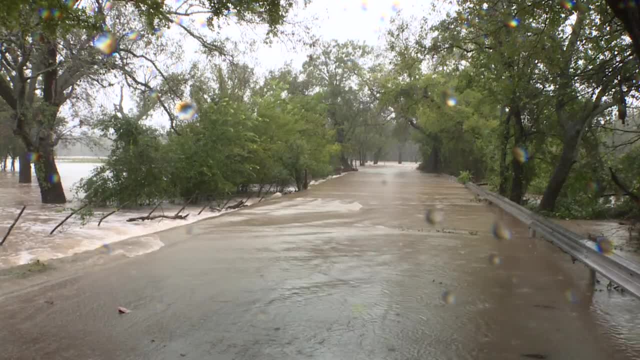 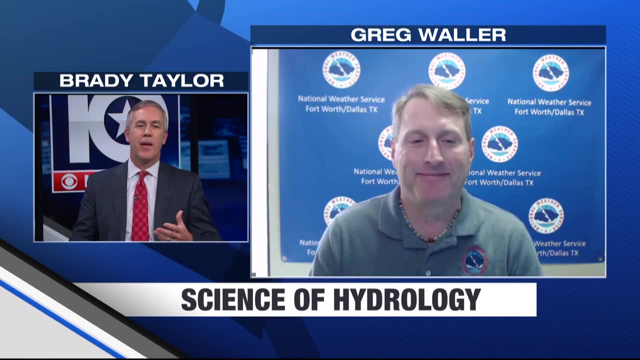 bit more, but it is critically important to make sure we stay situationally aware of our entire 400 000 square mile area. wow, 400 000 square miles. that is a lot to cover. so, off the top of your head, what were some of the big events of flooding events that you all had to to cover? 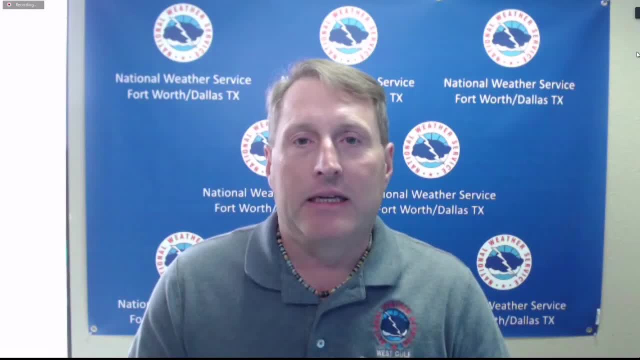 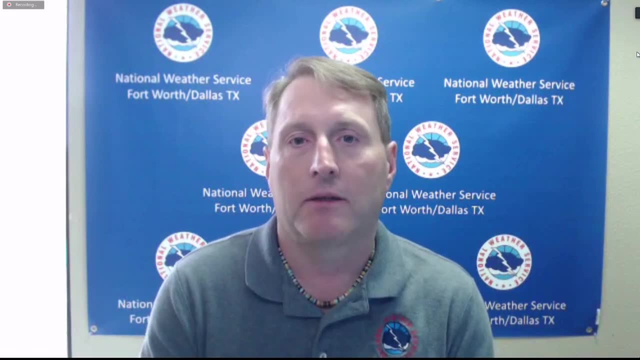 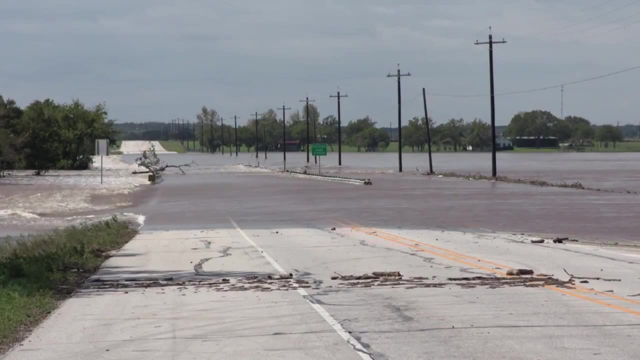 that's taken a lot of work in your office in in my two decades here at the river forecast center. the big one that everyone is going to lock into is harvey. uh in the houston area. uh, unprecedented impacts hitting a vulnerable, a very vulnerable population. if it wasn't for harold harvey, you know. 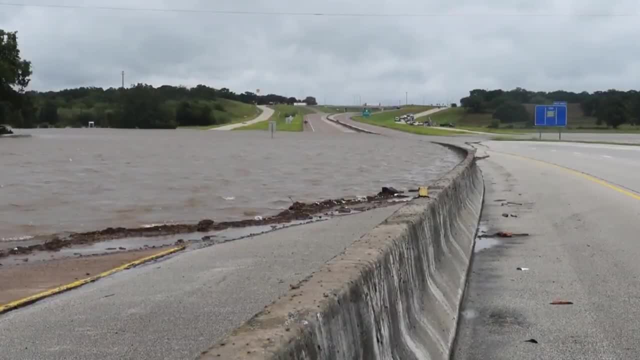 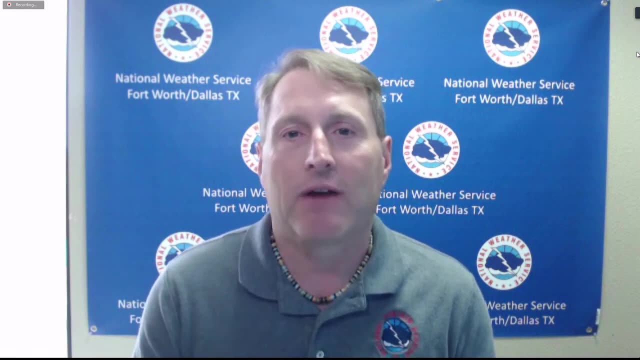 amelda, the following year would have been the talk of the storm that everyone was talking about from that extreme rain event, but the 2015 event, where almost the entire state of texas had a heavy rain event every single day in the state of texas had a heavy rain event every single day in the state of 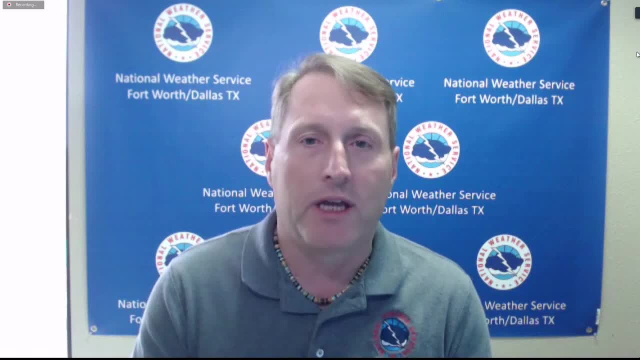 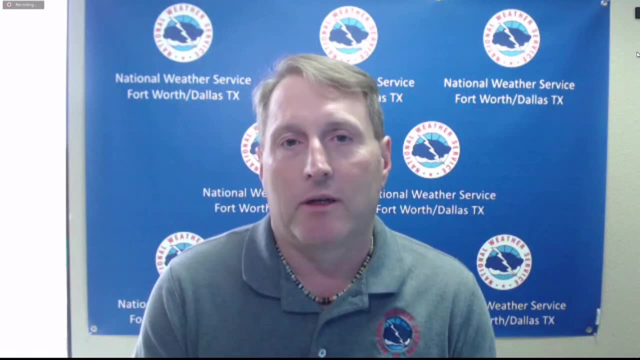 texas had a heavy rain event every single day in the state of texas had a heavy rain event every single day for a month. uh, the large scale events, uh, memorial day floods of 16. uh, the austin floods that were around halloween, uh, you know, there's so many of them. and one thing to point out: you know. 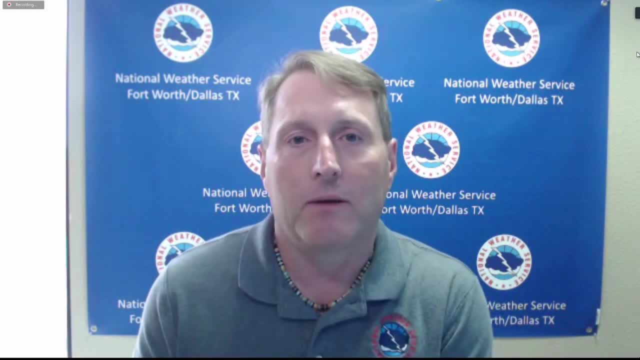 hurricane alex in 2010 was harvey before harvey. i mean, it was a large category three hurricane that moved inland, sat and dropped rainfall that that area never seen before and produced flooding on all day on the rio grande. so there are so many 2007 large events 2002. so 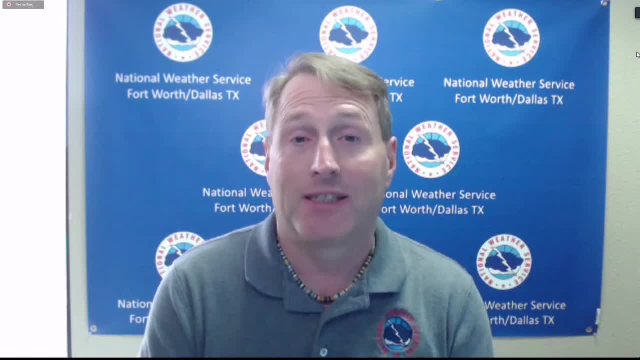 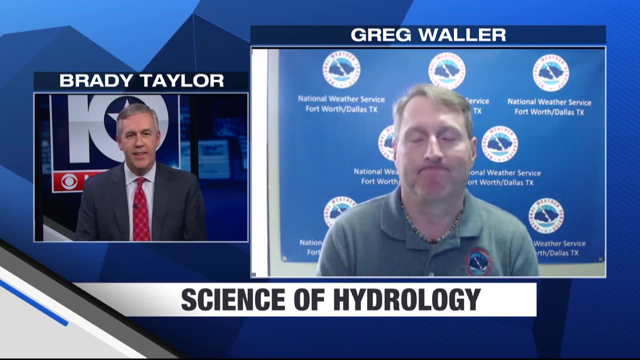 So, unfortunately, I've got a lot of significant flooding events under my belt. Wow, Yeah, I remember the 2016.. I was actually out chasing the storms and having to avoid some of that high water while we were out, And remember the river's coming up. 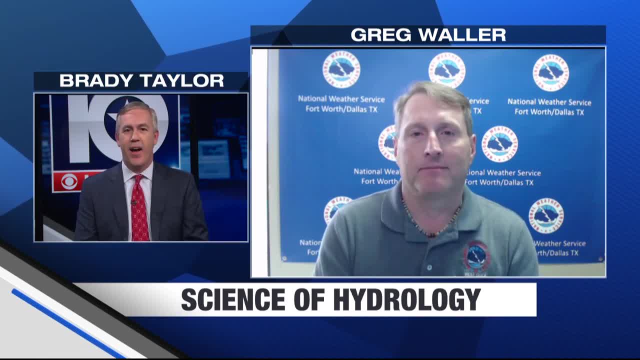 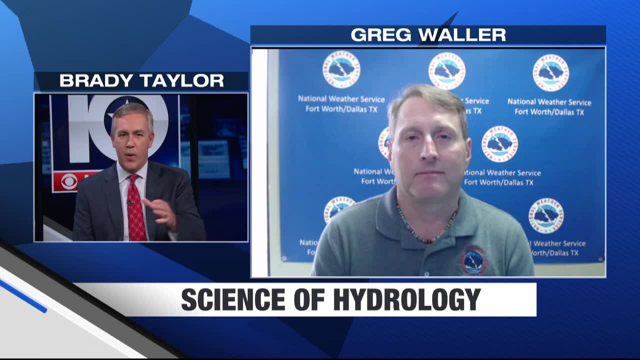 But it is crazy to think that we could see that and then still be extremely dry and hot like this. I can tell just by talking to you you're extremely interested and passionate about this. What got you directed into the science of hydrology? 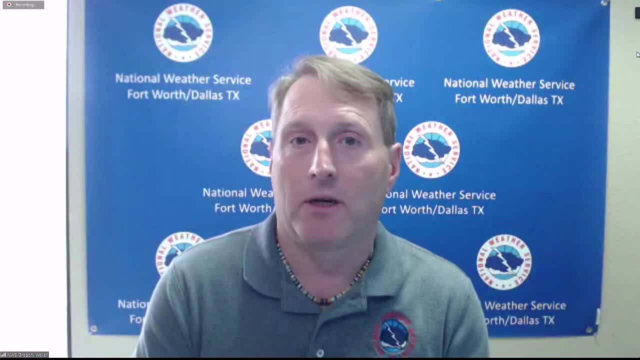 It started with a passion of meteorology. I'm a 13-year-old on the north side of Houston when Hurricane Alicia hit in 1983. And I want to know what is this power? What's going on? And I went to get my meteorology degree from Texas A&M University. 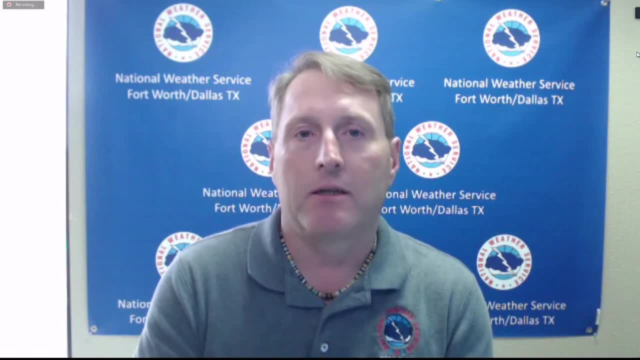 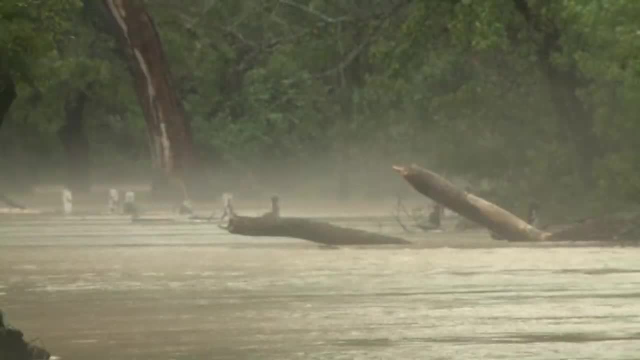 But once I joined the National Weather Service I noticed that flooding kills more on average. You know, on any four years, three years there'll be flooding will be more than tornado. Tornadoes get a lot of publicity, But I wanted 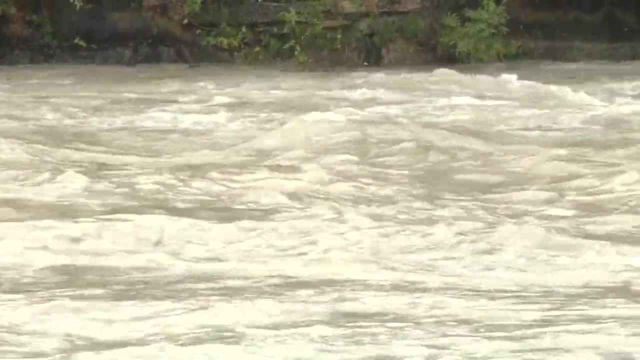 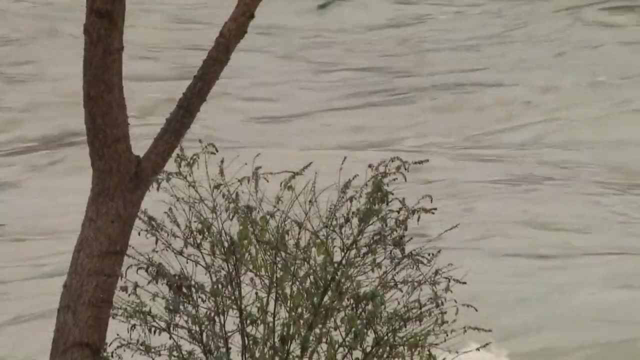 My passion was trying to figure out the flooding, especially Texas flooding. And when it jumped over into the river forecast in our world in 2000,, it started zoning in on just the volumes of water that Mother Nature can produce around here. And you know, I joke that Father Time is undefeated. 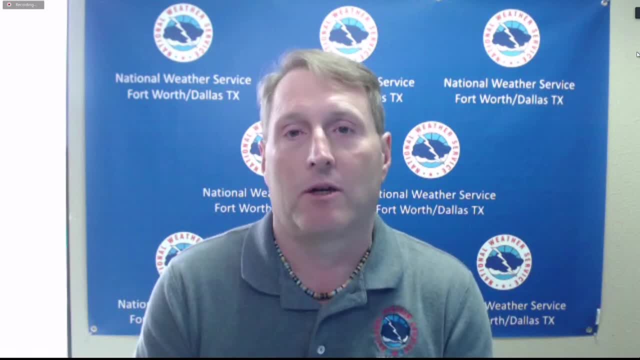 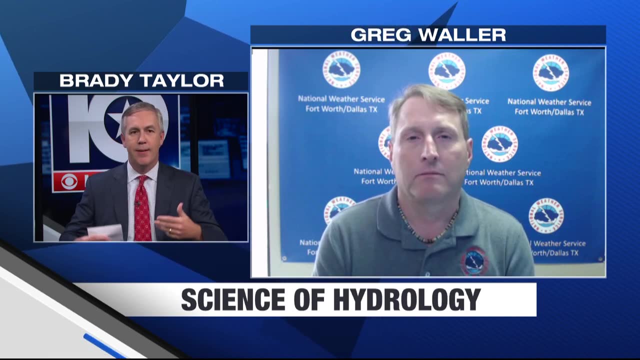 And I also joke that Mother Nature is undefeated. There's always something to learn, And you were talking about the number of deaths from flooding. What kind of advice would you give people when it comes to flood safety and preparedness and what to do? 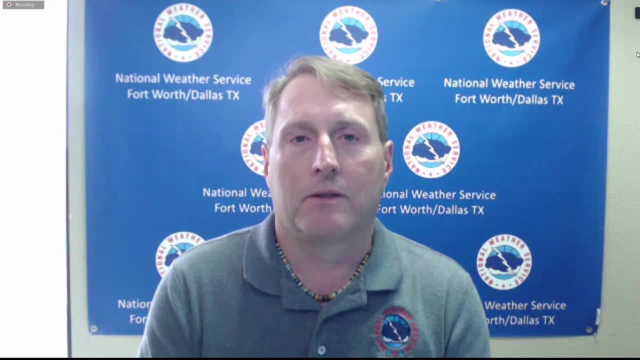 When we go through something like that. The first one: don't underestimate the power of water. I know this sounds kind of vague, but most of our stats show that we can probably eliminate half of our flood-related fatalities if we can keep people from driving through flooded roadways. 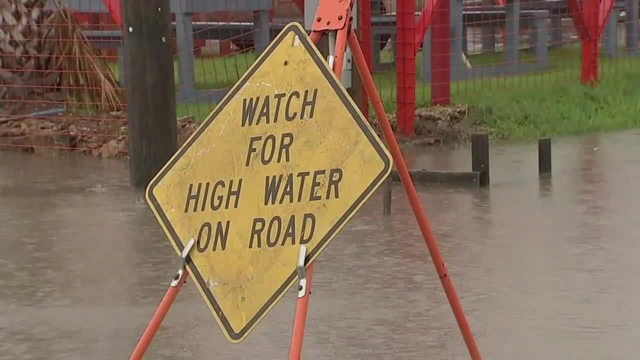 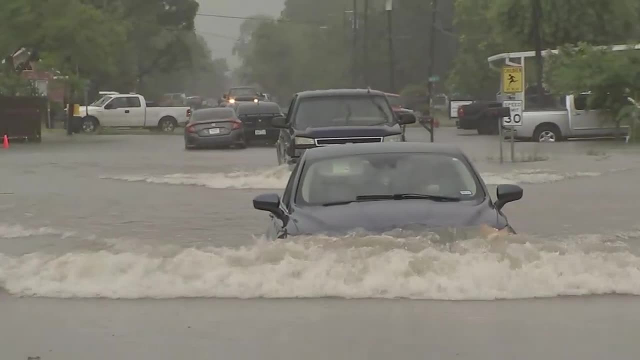 But you know, water's got a lot of heaviness to it And when it's moving it's got a lot of force to it. And you may think that you've got a big vehicle and can drive around it. But what I tell everyone, it doesn't matter how big your vehicle is. 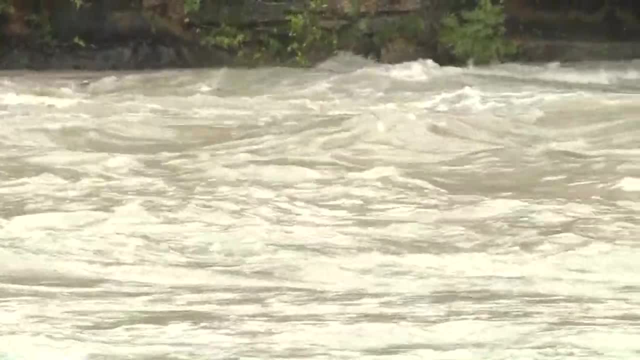 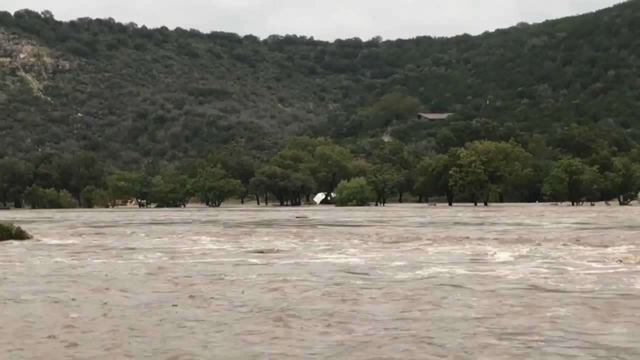 You know, the Titanic was a big vehicle. It floated And eventually it sank. And when you drive a vehicle into a flooded roadway and you lose contact and you start floating, you don't have a rudder, you don't have an engine and you're at the mercy of 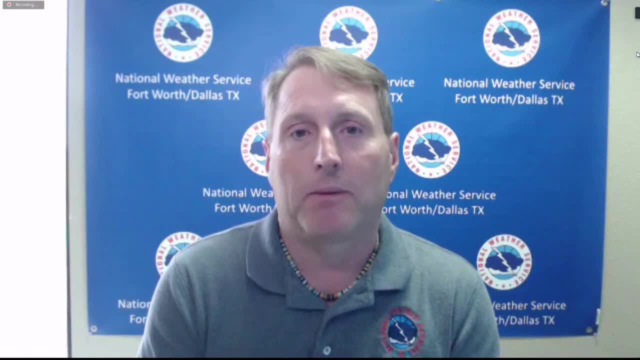 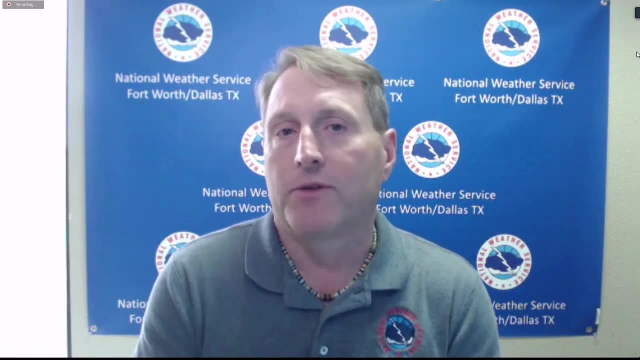 the water, And if we could just get that, there's probably half of our flood-related fatalities. The rest is if you know your flood risk and you hear a flood warning, the Weather Service has determined that's a life-threatening situation, Take the appropriate action. 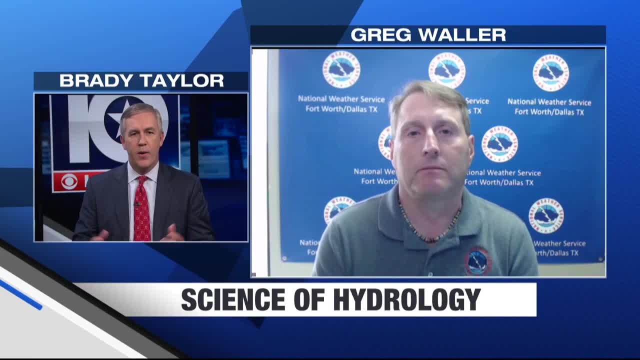 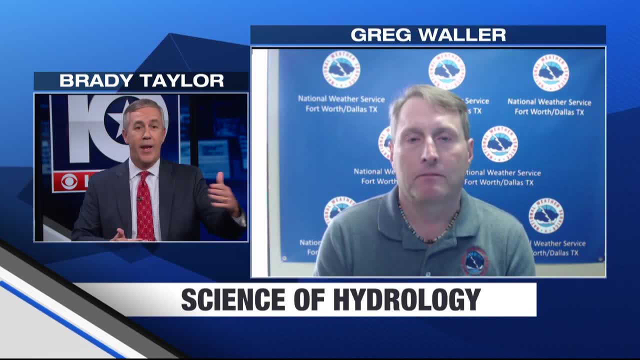 And the appropriate action is get to higher ground. So one thing that I always get questions on people was: you know, we'll have a big heavy rain event, You'll have your flash floods and stuff like that, But then the river flood warnings will last a lot longer. 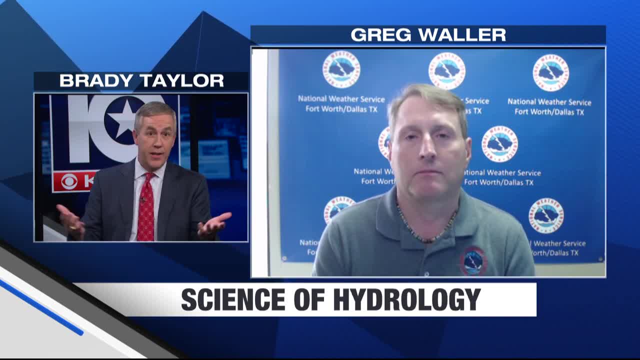 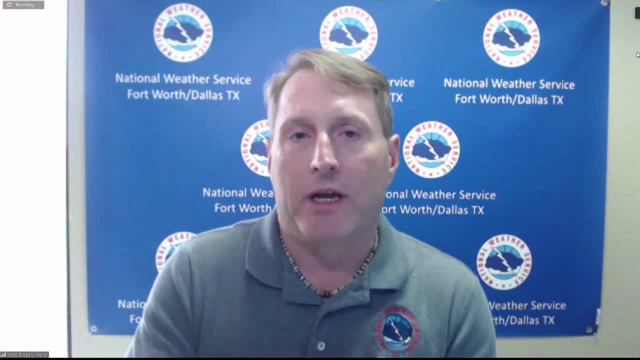 Explain how the runoff and the effects that has on the rivers, as they could keep rising after an event. The best way for me to explain it would be: you get rain locally in the Waco area or you get rain locally and say in Hillsborough, and it drains out. 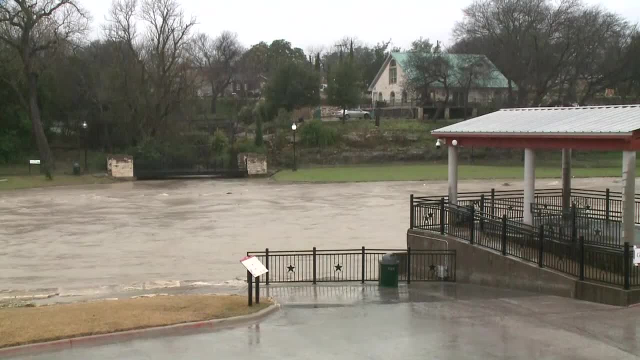 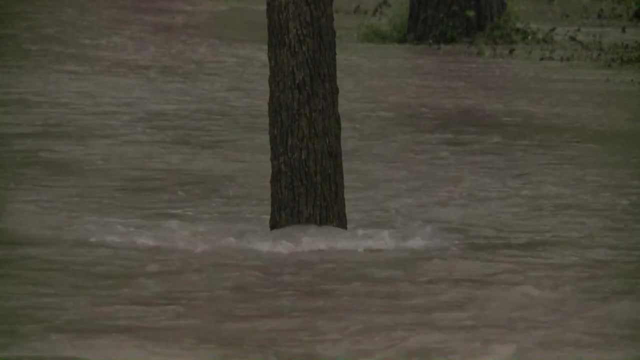 If there was a rain event upstream, that water's got to make its way through the system and come to you. So river flooding can be more long-term. A- because it may take the river longer to respond, But, B- there may be a flood event upstream. Do you know what's going on with the weather and the hydrology upstream that may cause that? A classic example of the Trinity River: when we have rainfall in the Dallas-Fort Worth area, it can take up to seven days to get down into the Lake Livingston area and then another seven days to get down to the mouth and Galveston Bay. 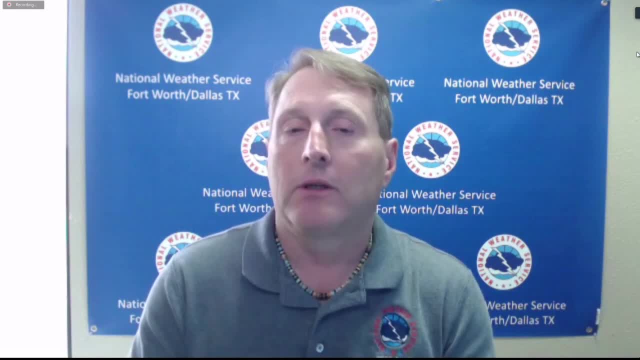 Local flash flooding. It rained hard on you or near you. It's a quick Moving system, But river flooding there's a lot that can go on, especially well upstream that could cause river flooding to hang around for days, if not weeks. 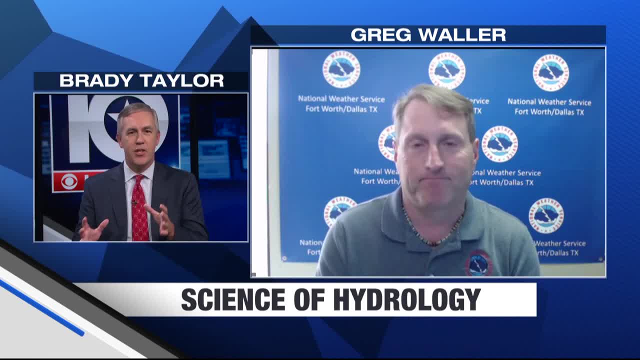 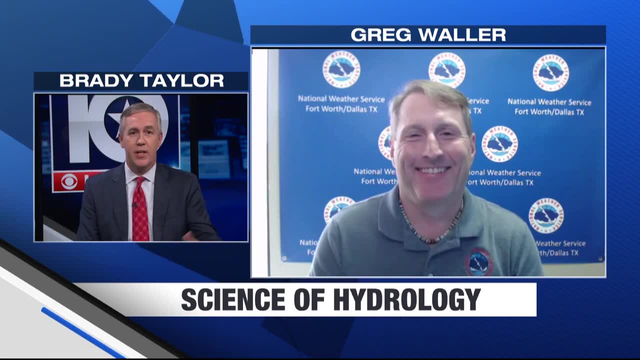 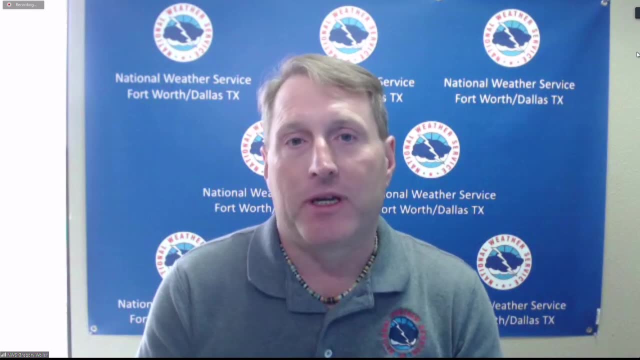 So you said you've been two decades of doing it. How much changes in the quality of forecast or have you seen? or just in the technicality of the forecast, with all the urbanization going on in the last two decades? From a weather forecast standpoint, when I first joined we did a three-day forecast from the National Weather Service and like a day four, day five. 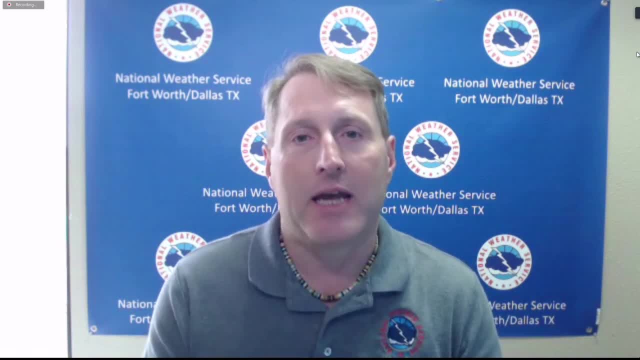 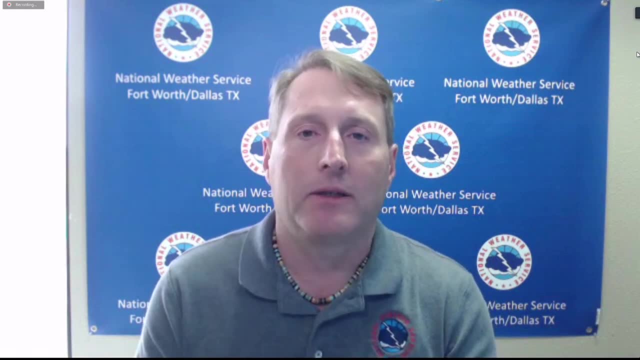 And now we do a seven-day forecast and the accuracy you know in that timeframe. we're probably more accurate now at seven days than we were three days back, you know, in the mid-90s. One thing that I do know is that you know our ability to forecast the exact rainfall amount and timing. it's called the quantitative precipitation forecast. 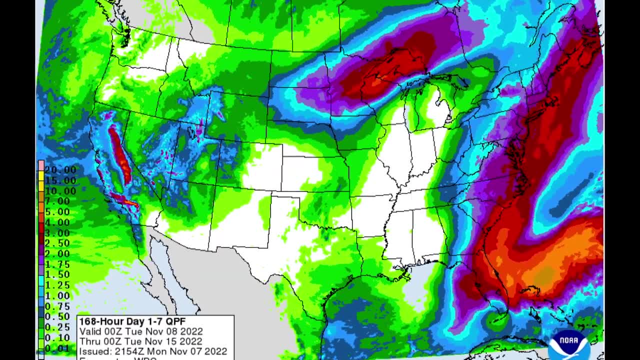 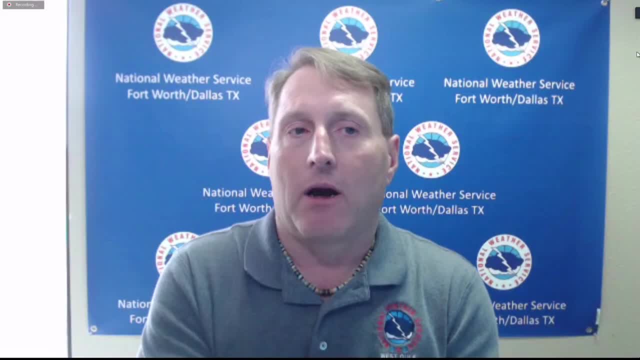 It's not a 30% chance of rain or scattered showers. It is saying the storms will develop here and produce this much rainfall in this timeframe And when I first joined, we did a three-day forecast And when I first joined, our weather models in Texas zero to six hours of lead time. 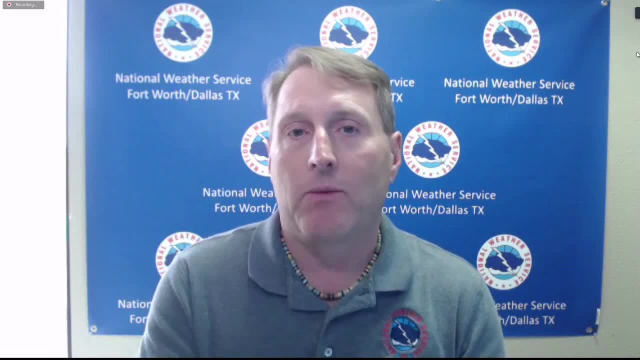 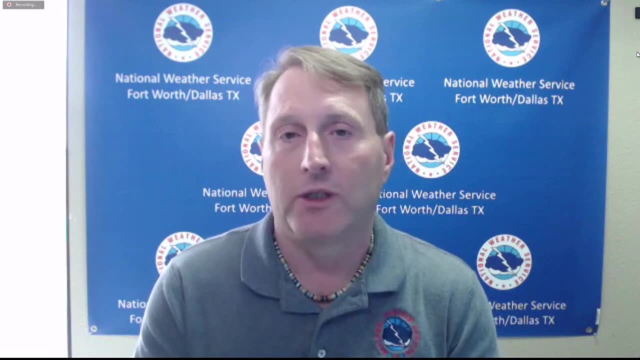 I mean, it really wasn't a lot. We can see a storm system coming in now and we get an idea that there's going to be a rain event, but we can expand that to 24 hours. The high-resolution meteorological models have done a really good job of expanding the accuracy of that forecast. 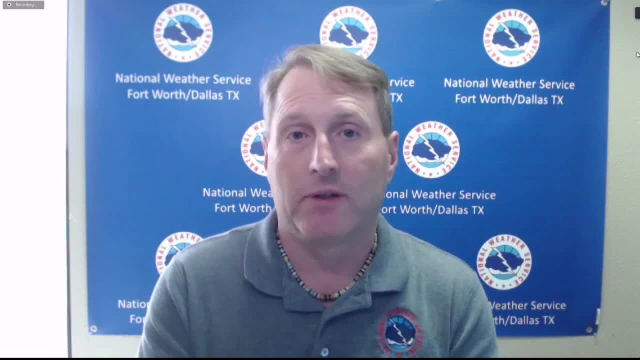 You give me a better rainfall forecast and my river forecasters will definitely give you a better river forecast, And we are, you know, smaller timescale, more resolution, And we're going to be able to do that in the next couple of weeks. 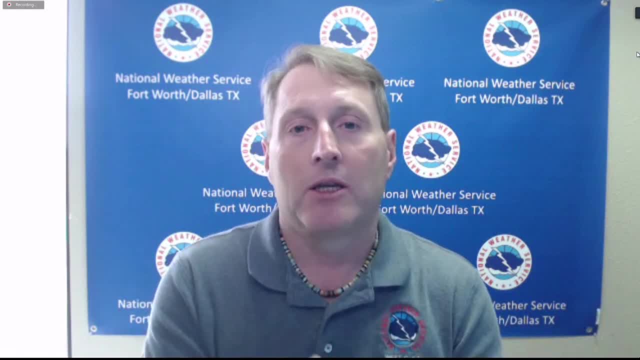 And we're going to be able to do that in the next couple of weeks because we have computing technology that allows us to go from a daily time step to a six-hour time step. So in some cases we have a one-hour time step on our river models to try to catch those peaks. 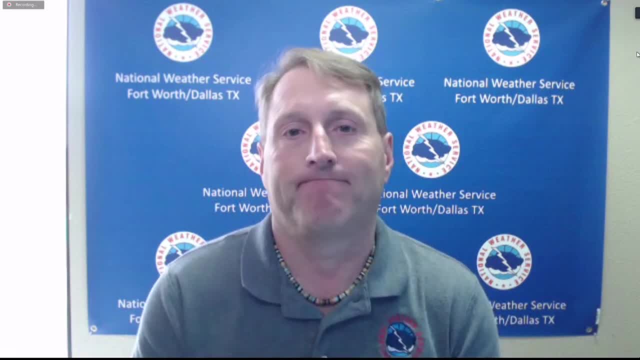 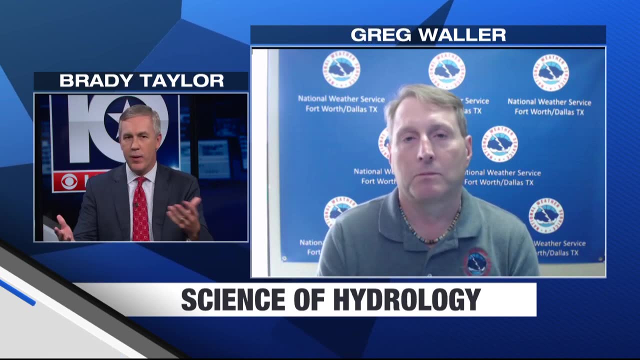 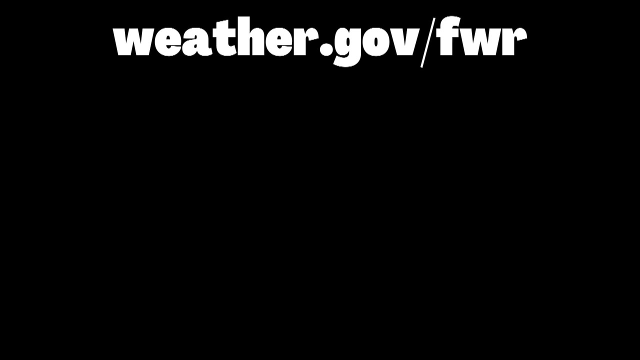 And that's computing, technology and science. Keep pushing, Keep pushing. That's awesome. So where can people find this, your stuff, from your office? if they wanted to find the data when events are happening like this, The quickest place would be weathergov. slash FWR Frank Whiskey Romeo. 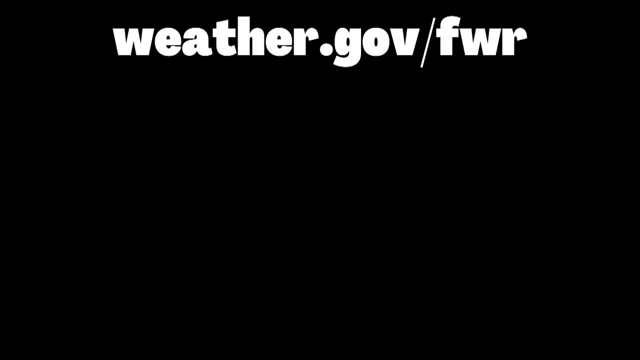 That would be the website. That would be the River Forecast Center page. The National Weather Service, River Forecast Centers and Weather Forecast Offices have their own pages. If you go, you'll see a map of Texas with all sorts of colored points.